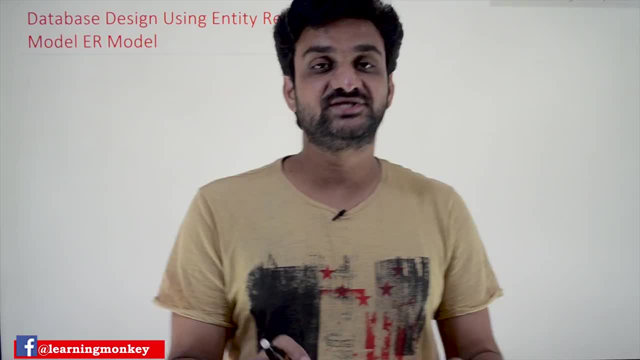 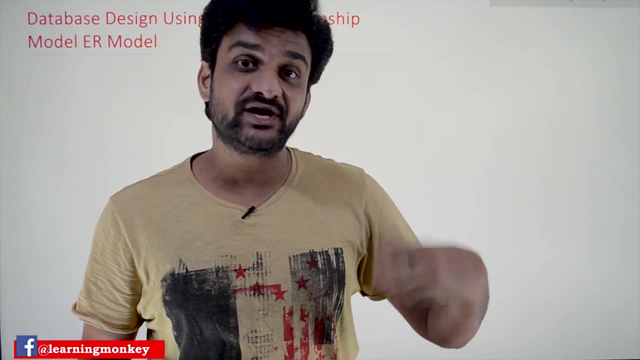 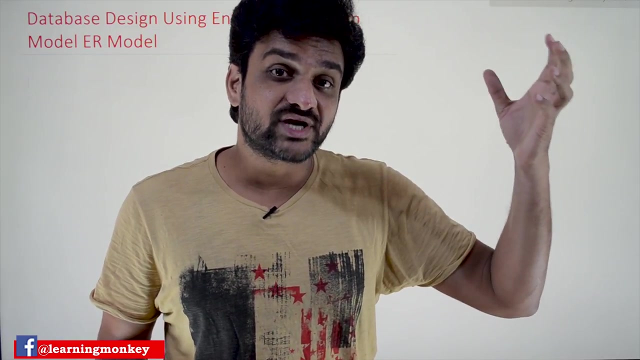 Will that happen in that way? No, What happens is, first we will go to an engineer and we will tell the engineer about the requirements of how we would like to construct our house, how we would like our house to be, So that those requirements are provided to the civilized. 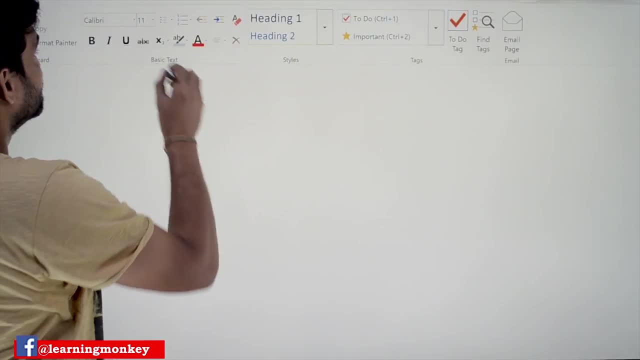 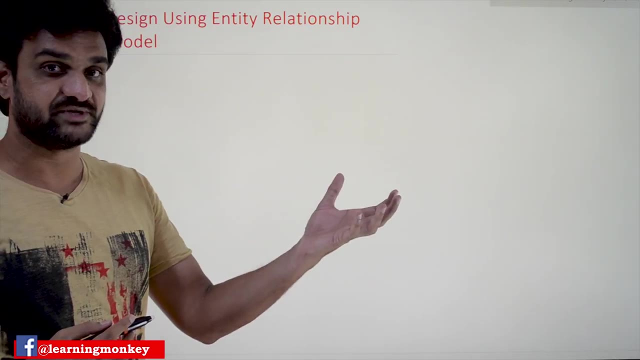 So let's try to understand that, For example, you want to construct a house and we have gone to the civil engineer and we have given our requirements. So what are those requirements are? First, we will provide the details of the sites. 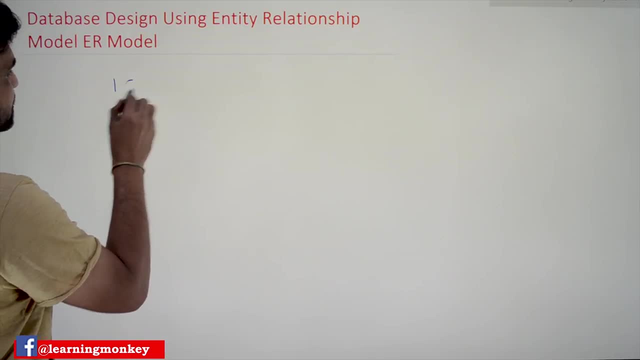 For example, details of the site. it is 100 feet length by 150 feet length width. So this is how the site will be. So this visualization has to be provided to the civil engineer Now. next, what we will do is we will give the requirements as three bedroom flat. 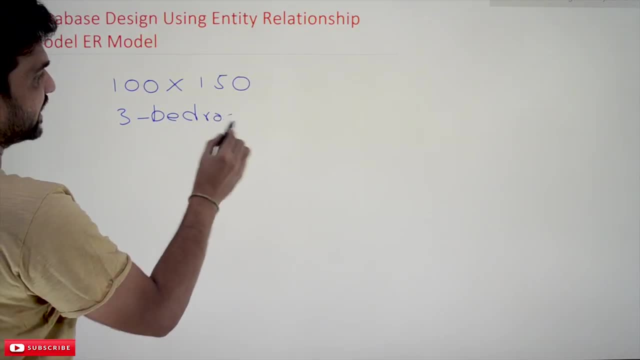 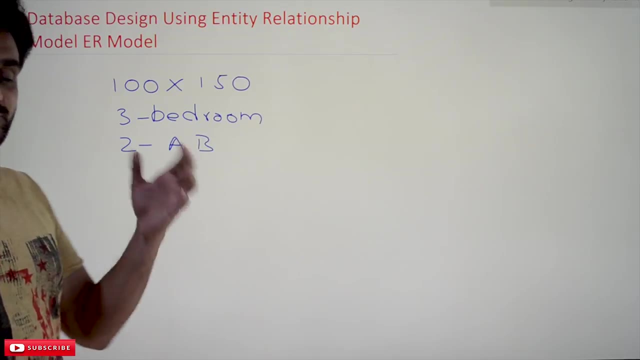 We would like to construct a three bedroom flat, So this is another requirement. and we ask two attached baths, So two attached bathrooms should be there. We need a parking space. Parking space is required. So these are all the requirements that are provided by the customer to the civil engineer. 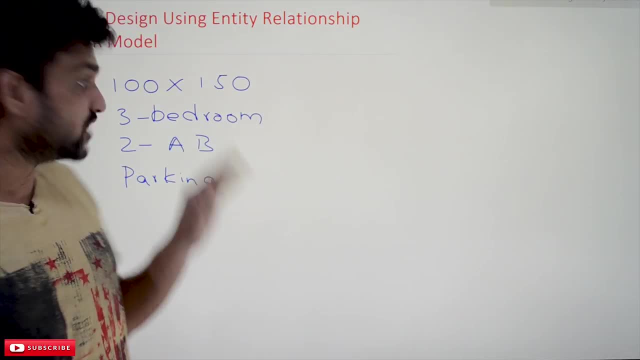 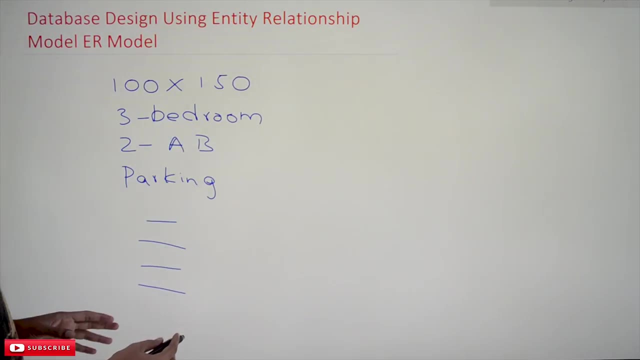 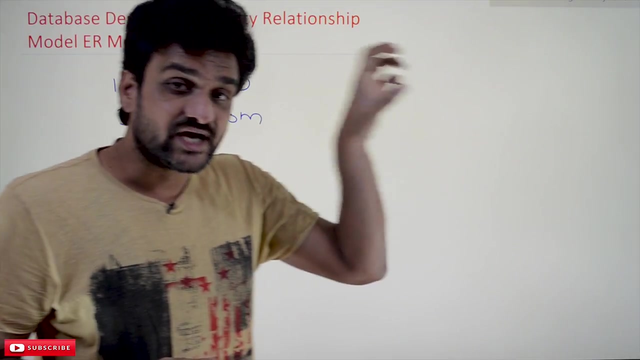 Now what the civil engineer will do. So, after taking all these requirements- so many requirements will be provided. After taking all these requirements- what the civil engineer will do is he will design this, So he is having some visualization. That visualization has to be put on the paper. 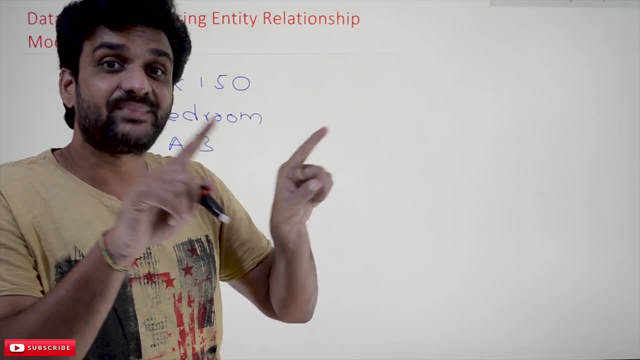 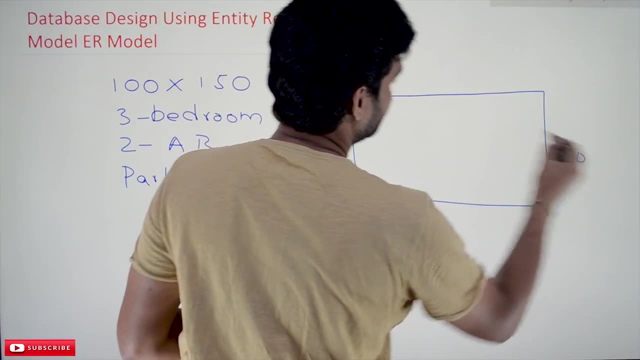 So for that to happen, he is going to give the plan, So he is going to take 100 feet length and 150 feet length. So this is 100 feet length, So this is 100 feet and this is 150 feet. 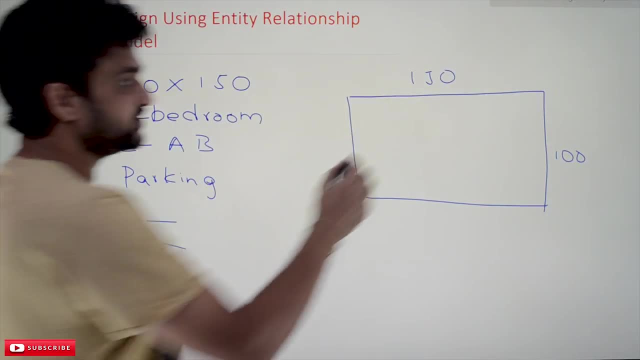 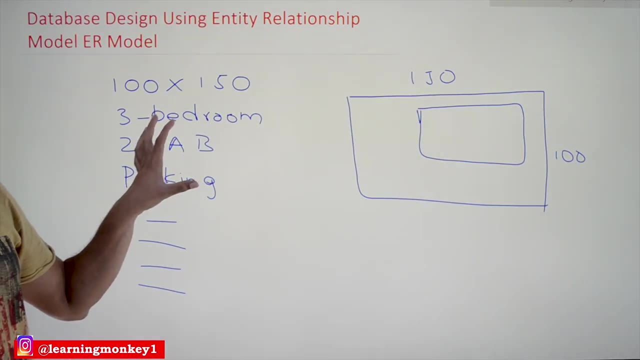 So with this he is going to get the visualization of the site. Now he is going to give the plan. So this is the house plan. So now this plan will be provided to the customer. This plan will be provided to the customer. 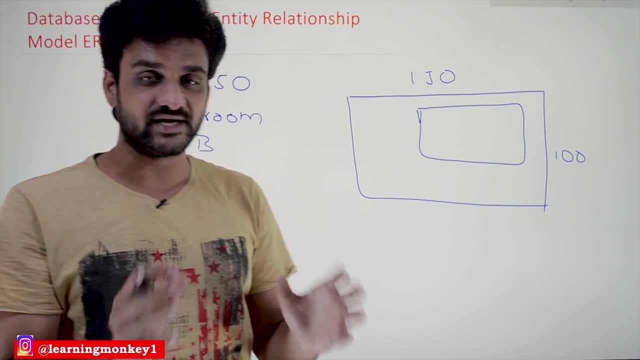 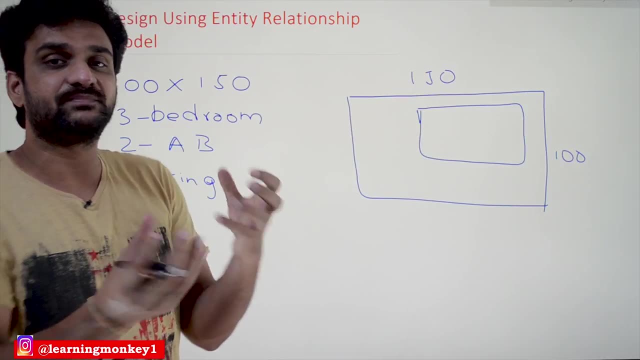 Now what the customer will do is he will verify all that content, So all that plan. he is going to check it clearly and he may give some another requirement. So, based upon that, the plan may change. And, finally, he is going to print the blueprint of the plan. 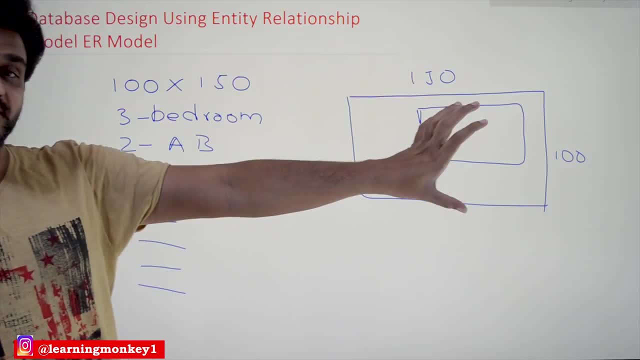 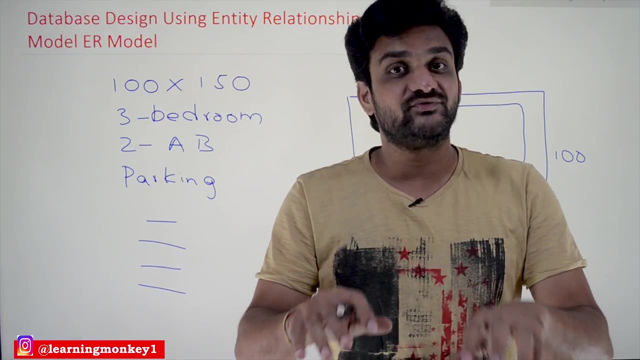 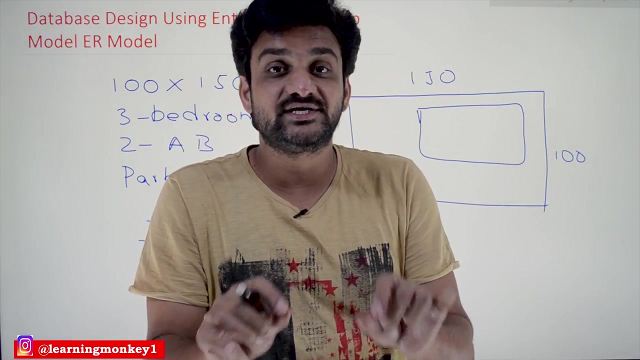 Blueprint of the plan. So, based upon that, based upon that blueprint, we will provide that blueprint to the constructor, And now the constructor is going to will construct the house based upon that plan. If you do the things in that way- that is what we call it as the construction of the house will be successful. 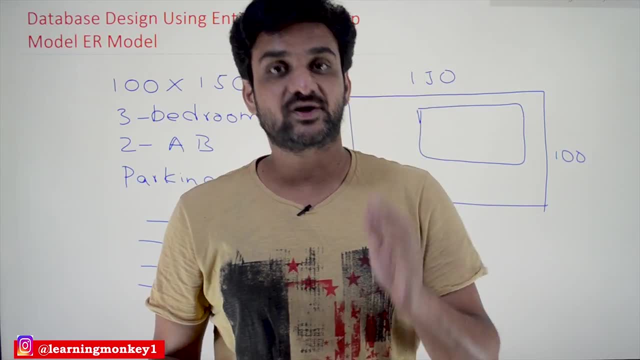 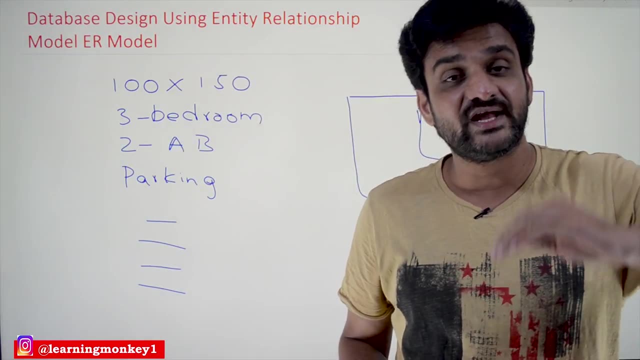 So the things will go according to the plan. Okay, So this is how the things will happen while constructing a house. So, in the same way, whenever we want to design a database, we have to collect the requirements, and for those requirements, 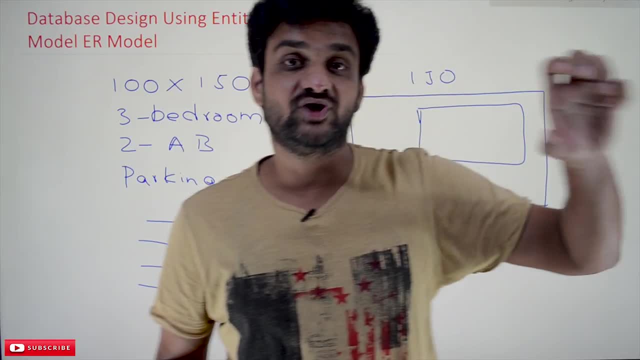 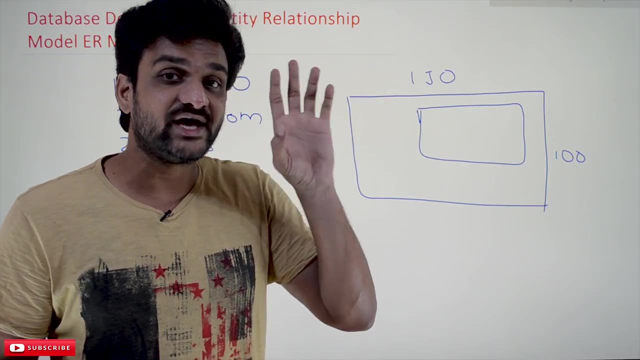 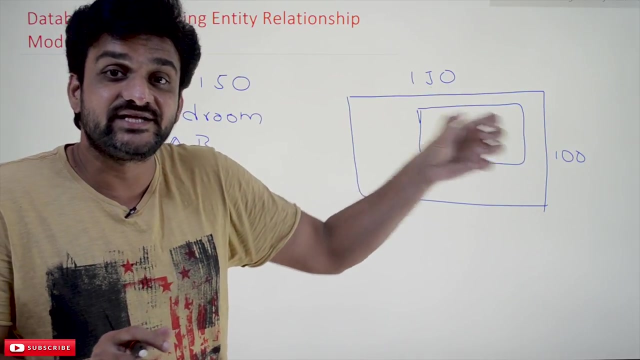 we have to design the database. So how the designing the database is done is it is done by using ER diagrams, As we know that the plan is done by using blueprints, So that plan, Similarly, similarly, the database design is done by using ER diagram. 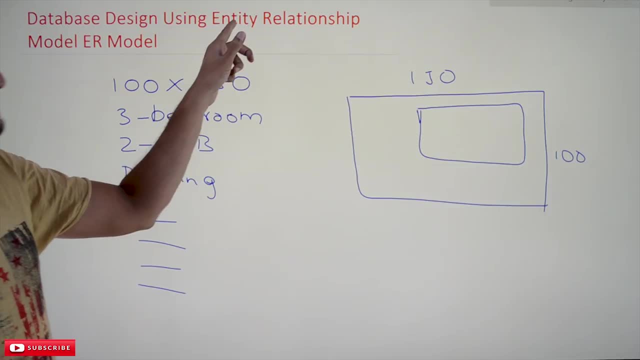 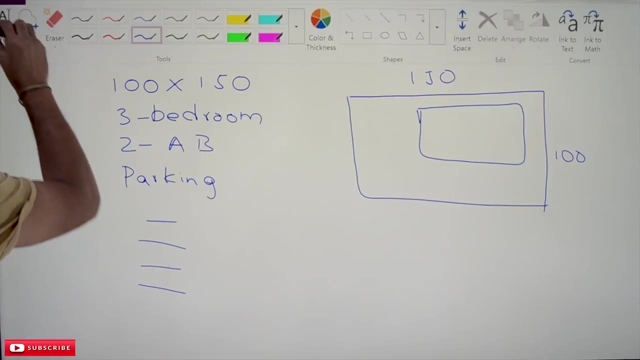 ER model or ER diagram So, which is what we call it as entity relationship model. So about these ER diagrams, we will try to understand. So this is how the design will be. For example, if you are asked to design a database, 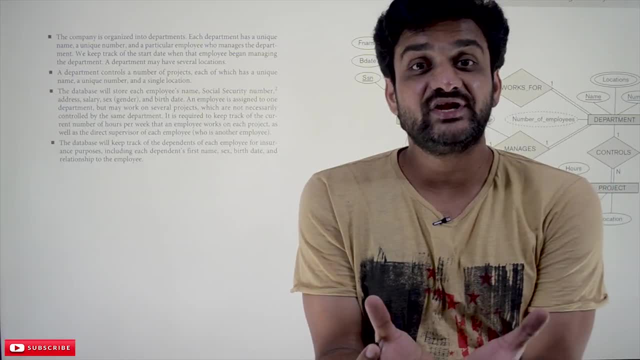 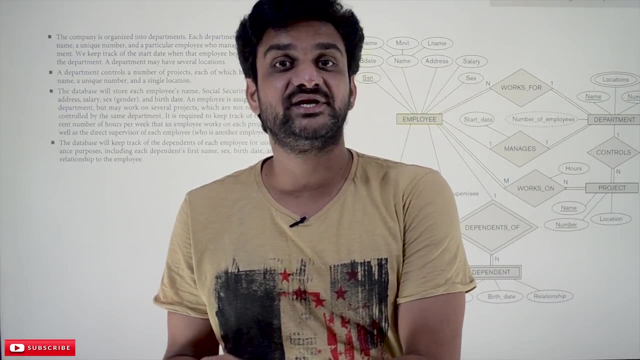 being an engineer. what we will do is: first, we will collect all the requirements from the company. Why we need to collect the requirements? Because we don't know what the company is, how they work and what kind of data they want to store, and what is the relationship between the different entities. 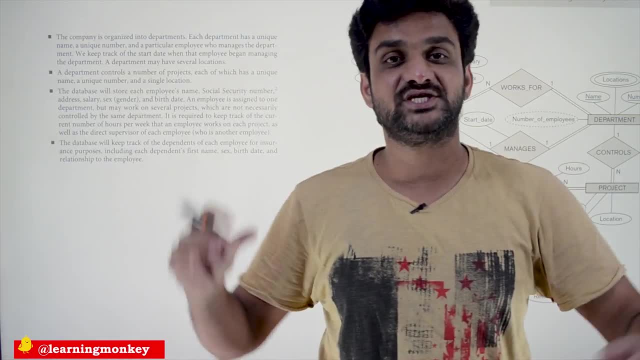 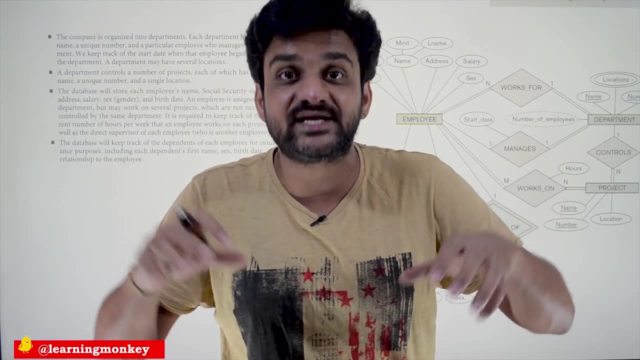 Different entities means departments, projects, employees. These are all what we call it as entities. So among these entities there is a relationship. So we have to find that relationship. and what are the different? we have to collect all the different possible collections. 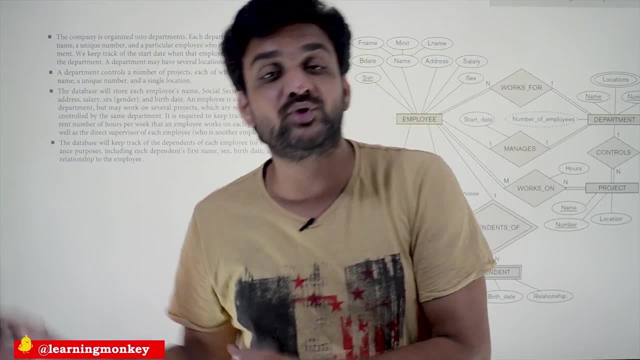 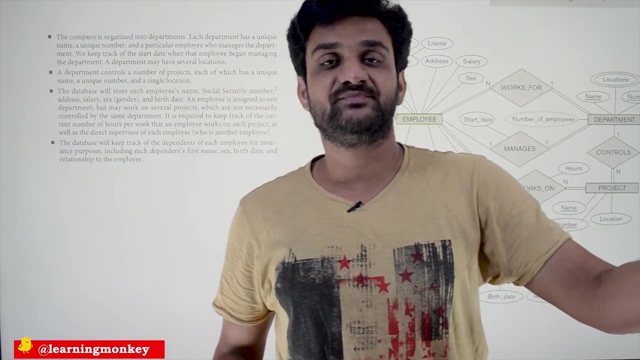 all the possible requirements that are there with the employees of the company. So we are going to go to the each and every employee, almost every employee. We will ask them: what kind of requirements do you need? So, based upon the requirements that we have collected, 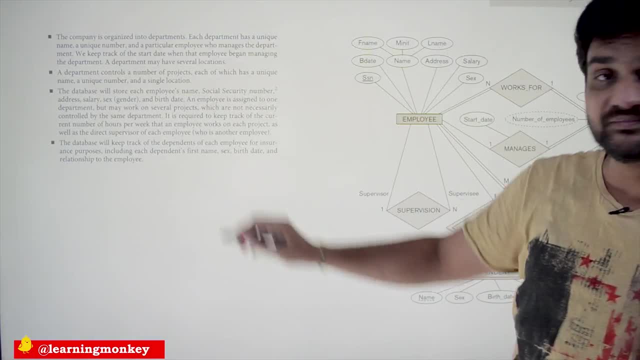 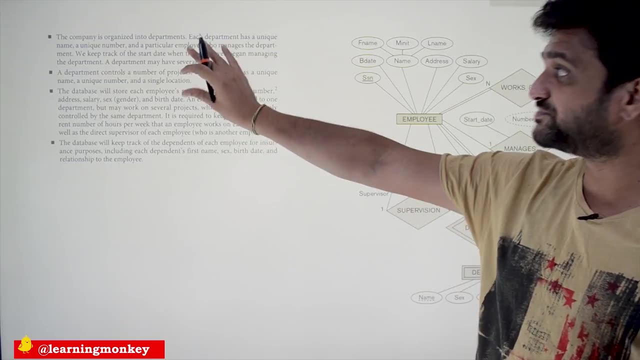 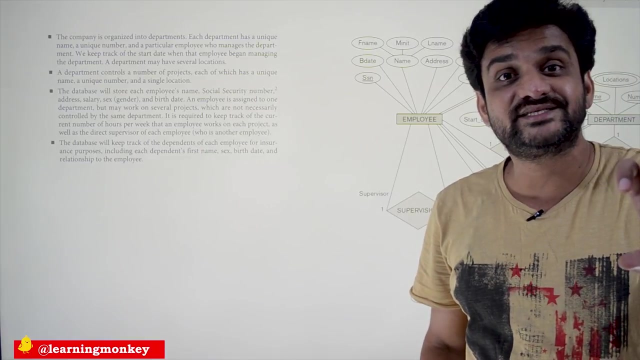 So, for example, assume that for this, for the company, we have collected these requirements. So these are the requirements which is documented on simple language by using a simple language. So, based upon these requirements, the engineer will will design a database model. 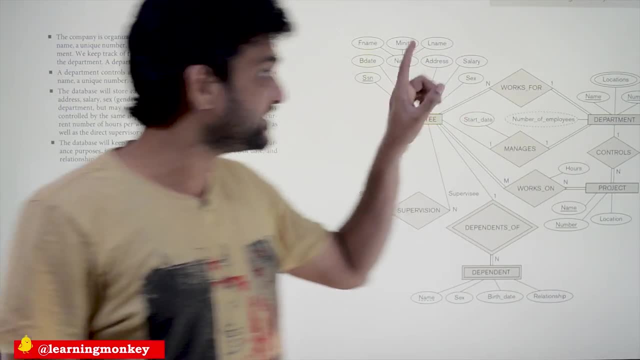 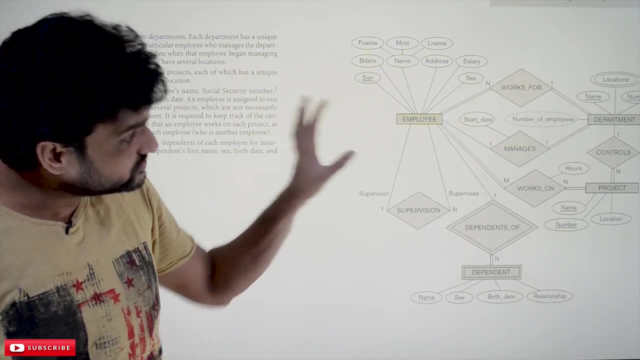 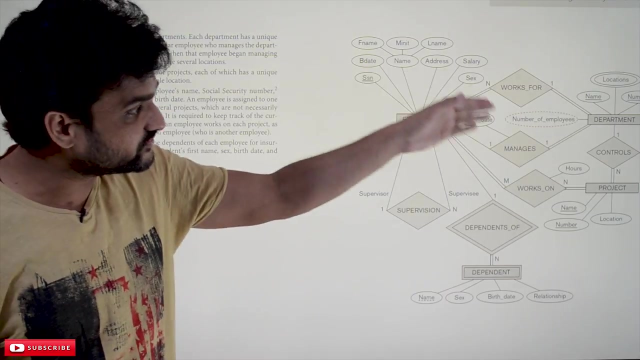 That design is done by using entity relationship model. So these requirements are converted into this, into this design. So how this design has to be done and how we are going to collect the requirement. So, after collecting the requirements, how we are going to convert these requirements into this diagram. 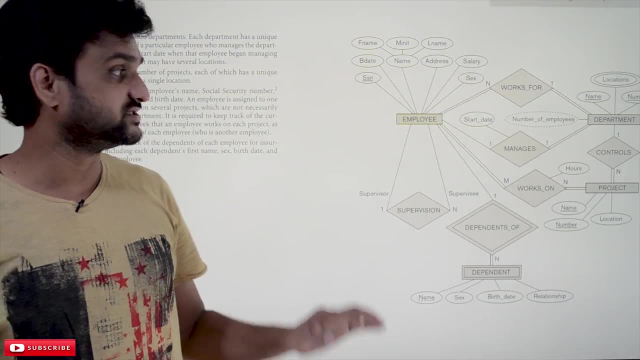 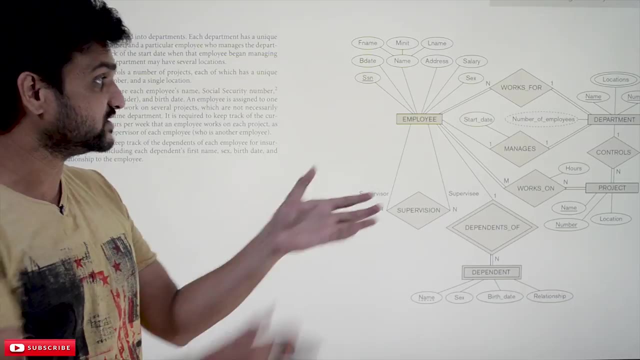 So how that is done, that we will try to understand in our later coming classes. So this is the ER diagram for the company database that we are going to design. So, after designing, so we will take this design to the software developers. 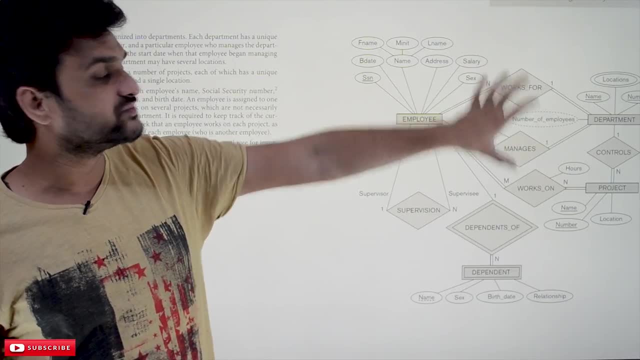 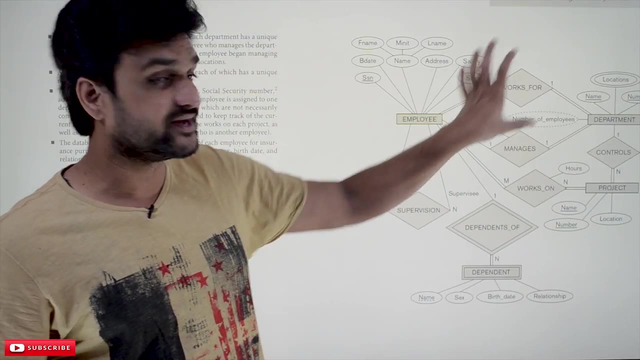 So what they will do is based upon this diagram. they are going to implement it on the computer. On the computer they will implement this diagram. So how that implementation will be done, that also we will see in our later coming classes. 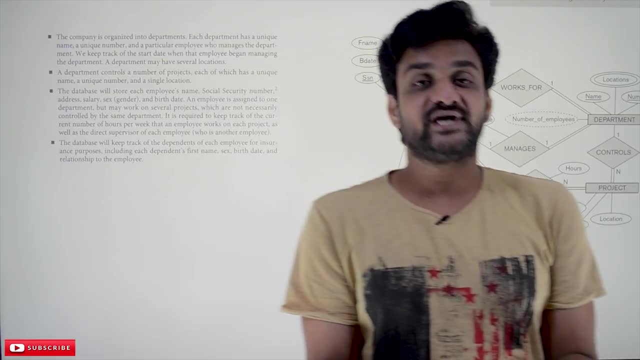 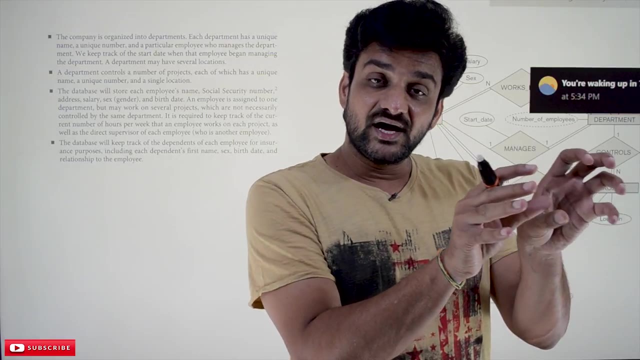 What you have to understand is, in order to design, we have to first collect the requirements and after that, based upon those requirements, we have to design the ER diagram. So, entity relationship diagram. Based upon that model, we have to construct a diagram. 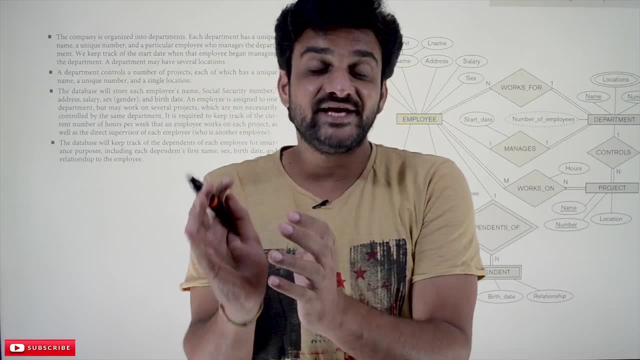 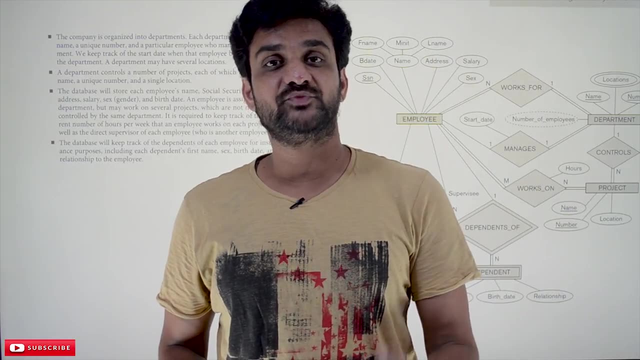 So this is the first phase of design of the database. After that the implementation is done. So this is all about entity relationship model. Hope you got the clarity on this concept. Thanks for watching. If you haven't subscribed to our channel. 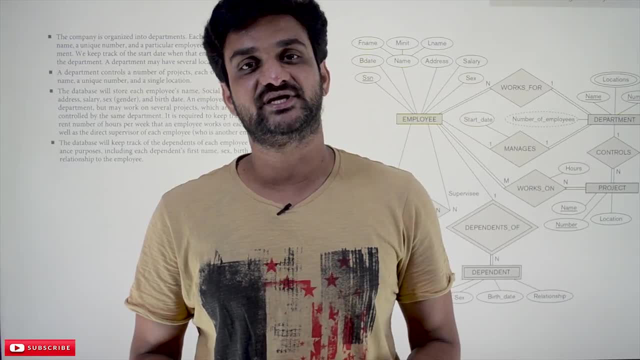 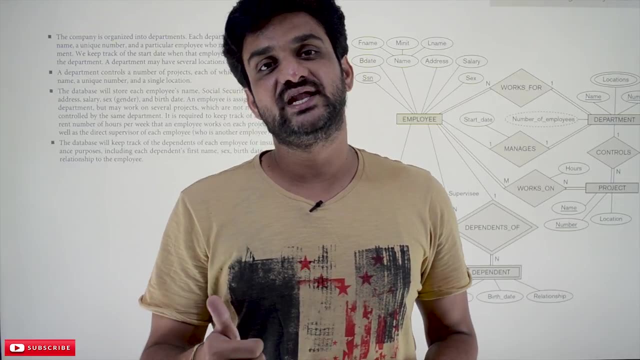 please subscribe to our channel and press bell icon for the latest updates. And if you have any doubts regarding this concept, please post your doubt in the comment section below. And if you feel that this video is helpful to you, please give us a like symbol.